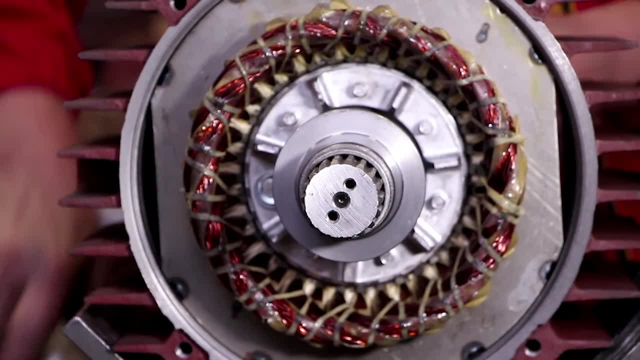 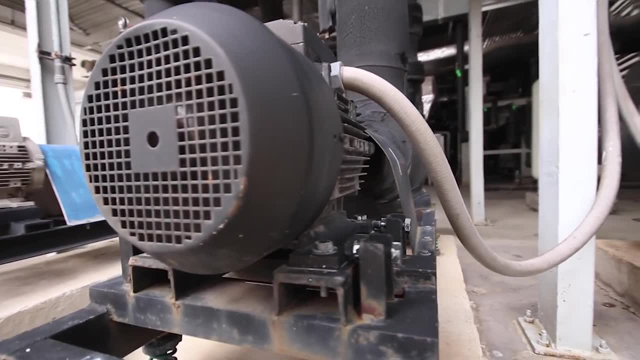 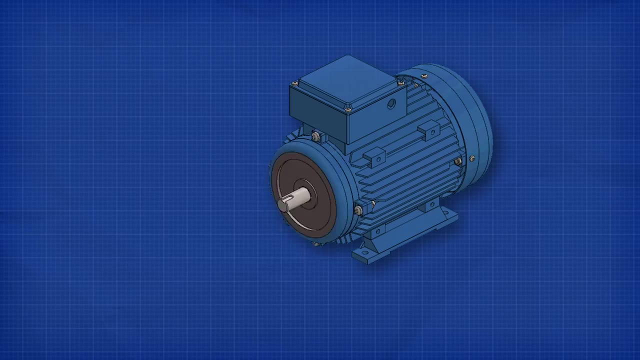 This is an electrical motor. It's one of the most important devices ever to be invented. These motors are used everywhere, from pumping the water we drink to powering elevators and cranes, even cooling nuclear power stations. So we are going to look inside one and learn in detail. 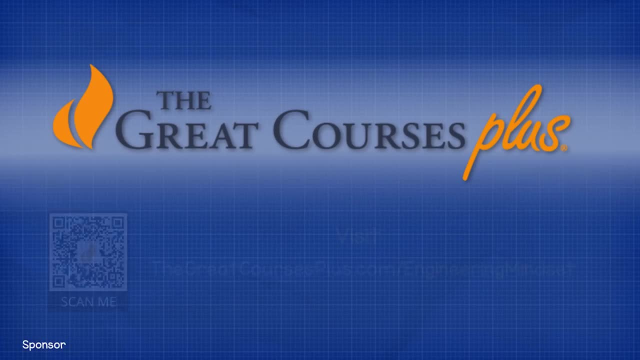 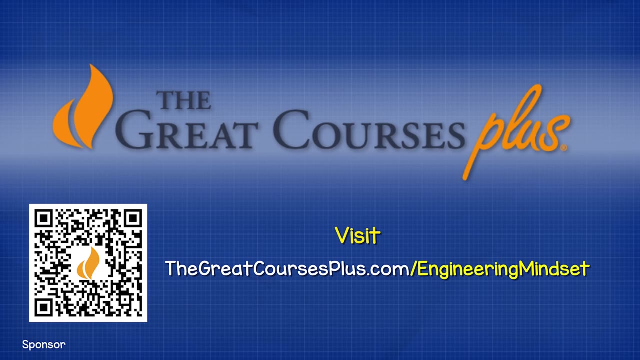 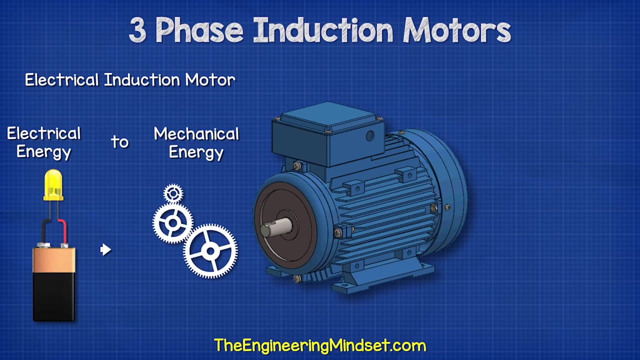 exactly how they work in this video, which is sponsored by The Great Courses Plus. Visit the link in the video description to start a free trial and get access to some truly great online courses. The induction motor will look something like this. They turn electrical energy into mechanical energy which we can use to drive pumps. 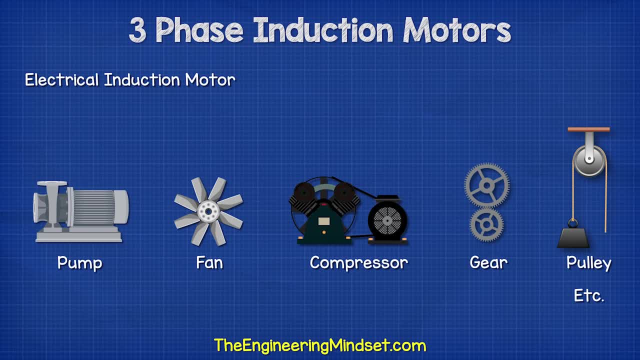 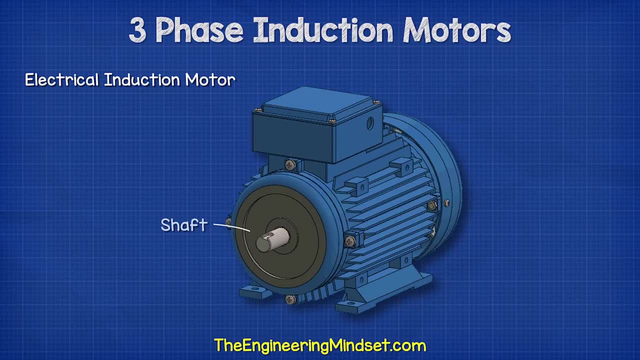 fans, compressors, gears, pulleys, etc. Almost all the parts are held inside the main housing. At the front we find the shaft. This is the part that rotates and we can calculate the amount of energy that is produced by the shaft. 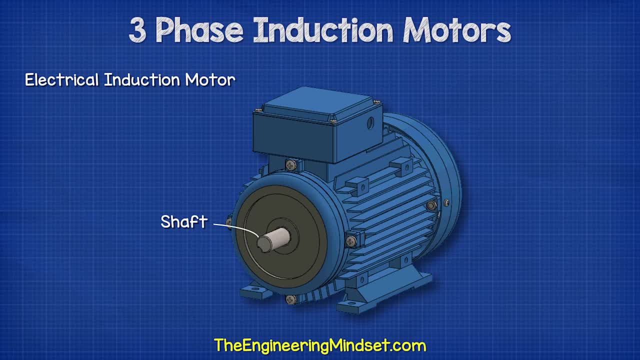 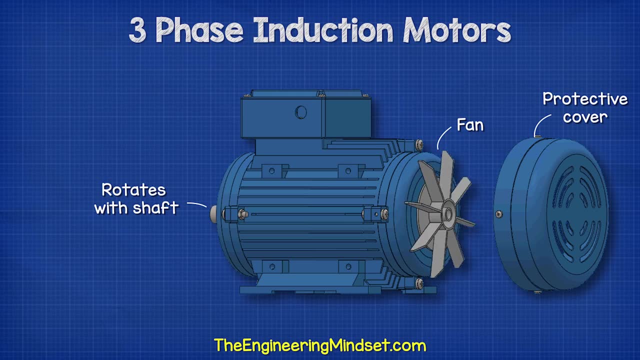 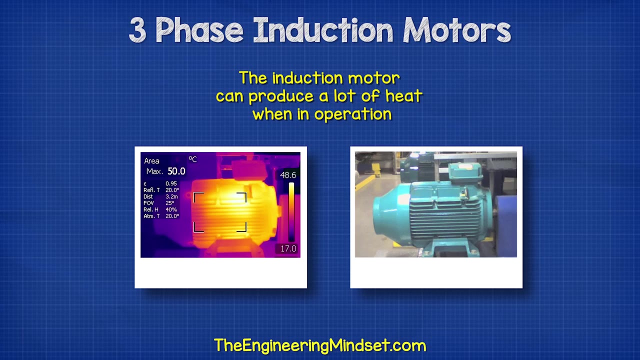 We can connect things like pumps, gears and pulleys to this to do work for us. At the back we find the fan and a protective cover. The fan is connected to the shaft and so it rotates whenever the motor operates. That's because the induction motor can produce. 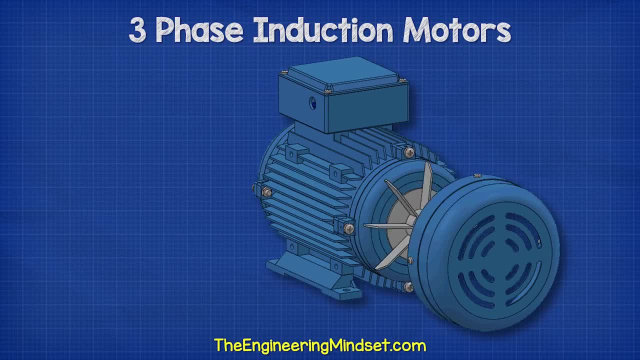 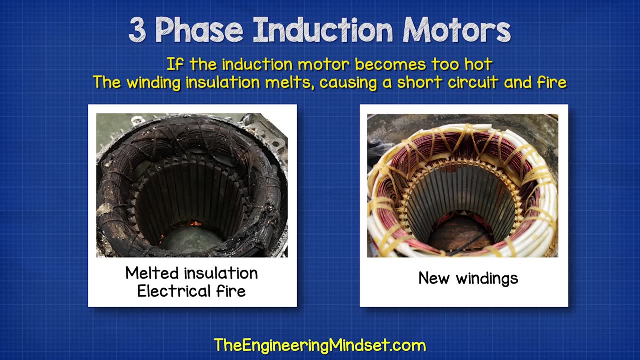 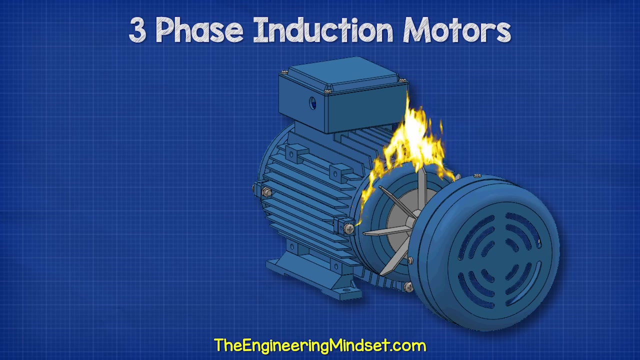 a lot of heat when in operation, so the fan blows ambient air over the casing to cool it down. If the induction motor became too hot, the insulation of the internal electrical coils will melt. This will cause a short circuit and the motor will destroy itself. The fins on the side of the enclosure. 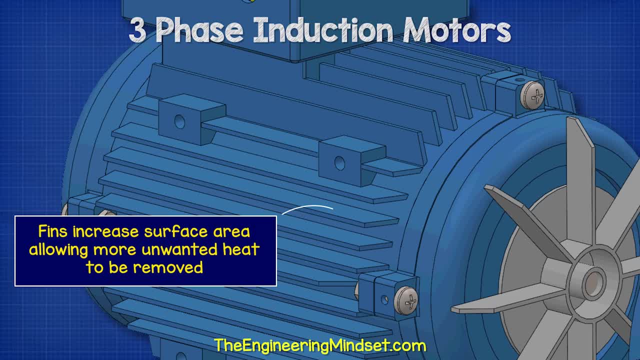 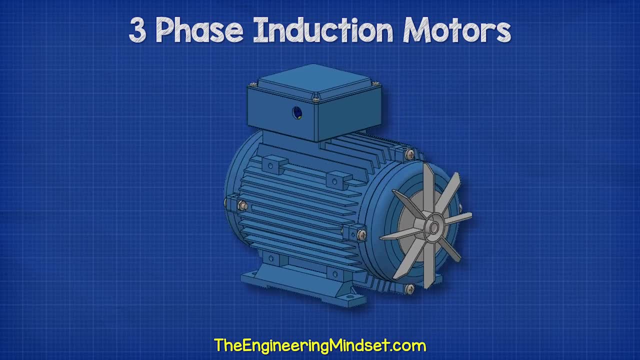 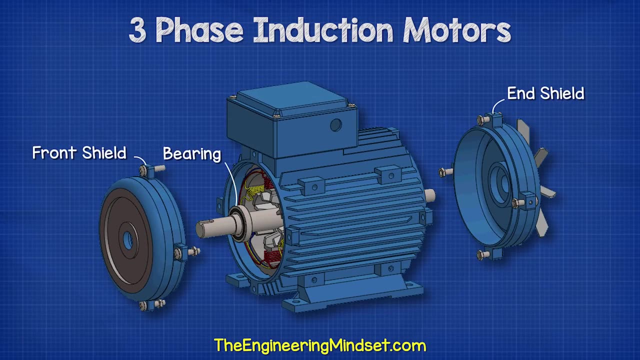 help to increase the surface area, and that lets us remove more unwanted heat. The shaft is supported by some bearings which sit inside the front, as well as the rear shields. The bearings help the shaft rotate smoothly and also hold it in position Inside. the shaft is supported by some bearings which sit inside the front as well as the rear. 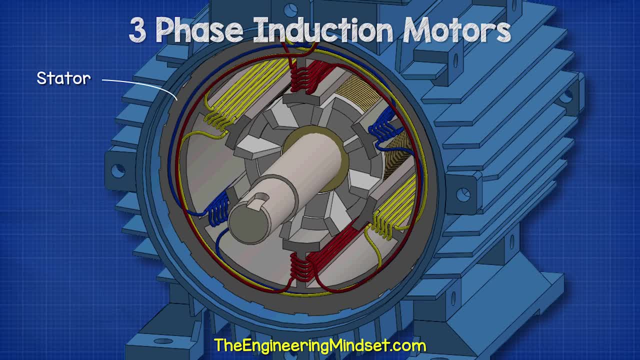 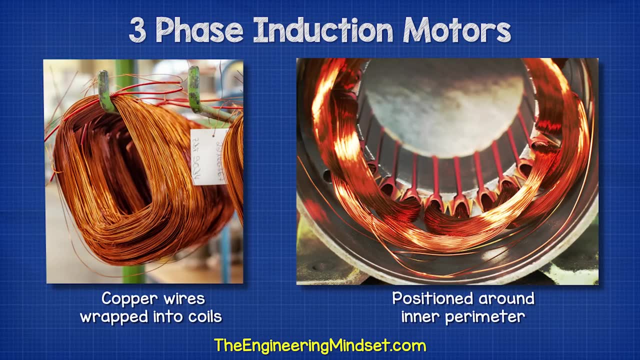 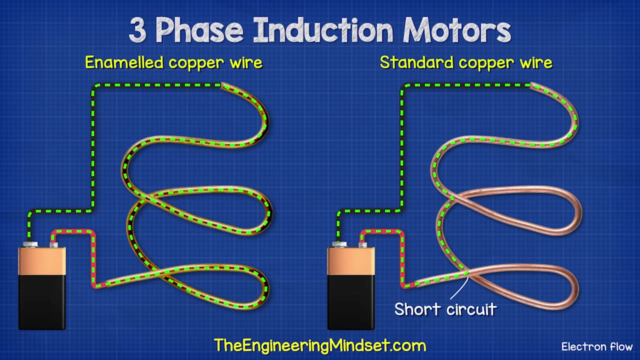 The bearings help the shaft rotate smoothly and also hold it in position housing we find the stator. The stator is stationary and does not rotate. This consists of a number of copper wires which are wrapped into coils between the slots positioned around the inner perimeter. The copper wires are coated with a special enamel which electrically insulates. 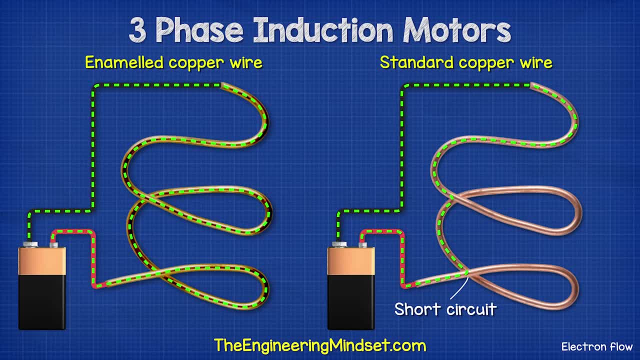 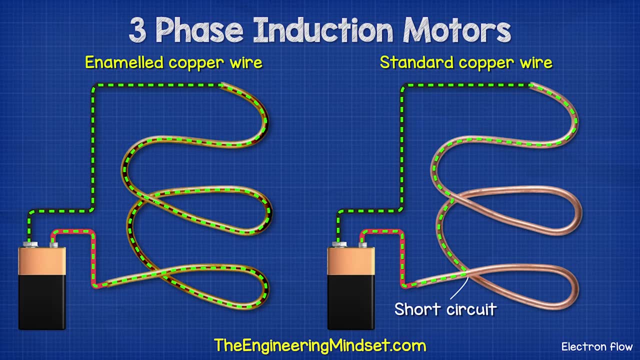 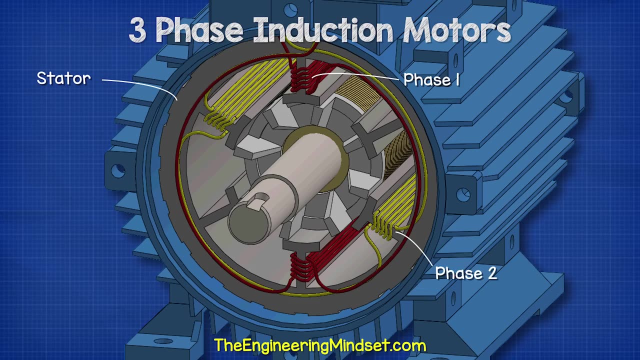 the wires from each other. This means electricity has to flow through the entire coil, otherwise it would take the shortest path possible, and we'll see why that's important a little later in this video. Now, this is a three-phase induction motor, so we have three separated sets of coils in the 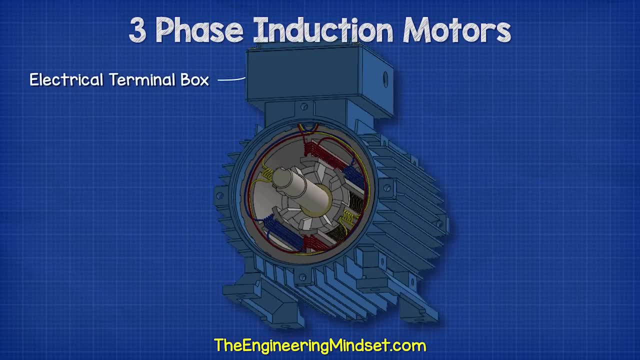 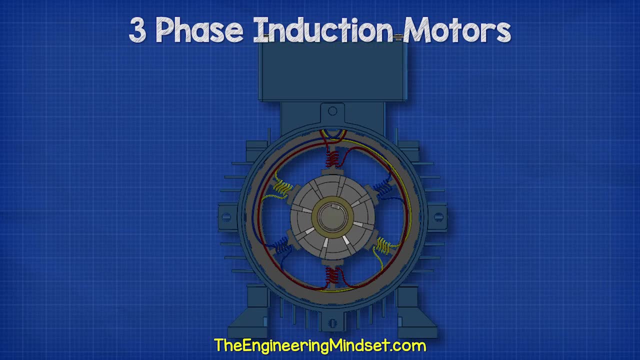 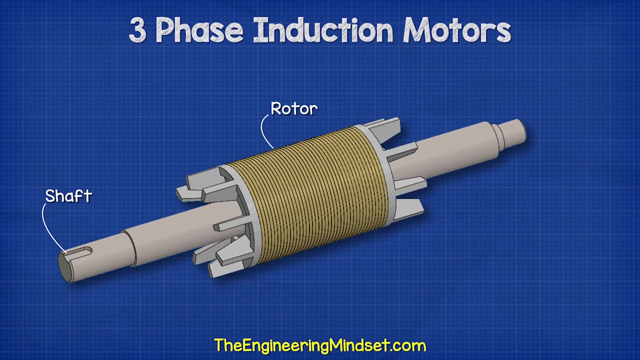 stator. The ends of each set will connect with the terminals within the electrical terminal box. We will also see how these are connected a little later in this video. When connected to the electrical supply, the stator generates a rotating electrode. Connected to the shaft is the rotor. In this case it's a squirrel cage type rotor. It's called a squirrel. 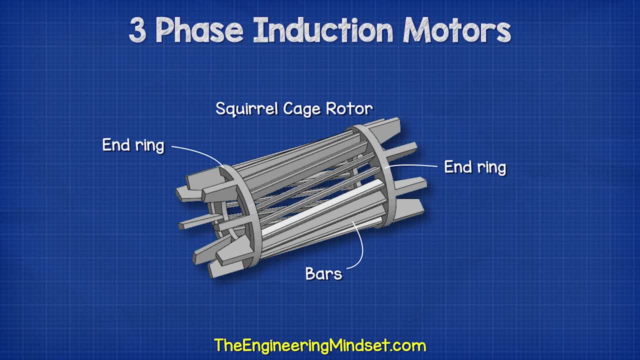 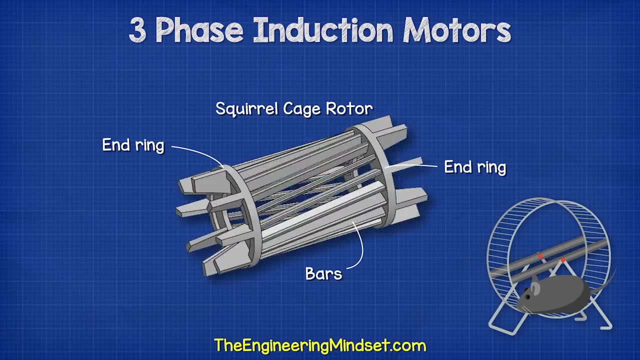 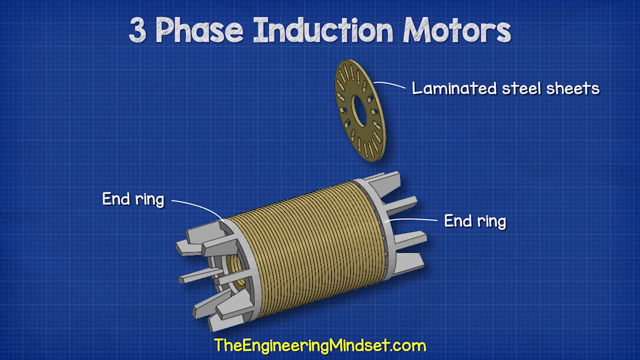 cage because it has two end rings which are connected by some bars, and these will all rotate together. This design is similar to a small cage or an exercise wheel used by a pet hamster or even a squirrel. The squirrel cage is fitted with a number of laminated steel sheets. 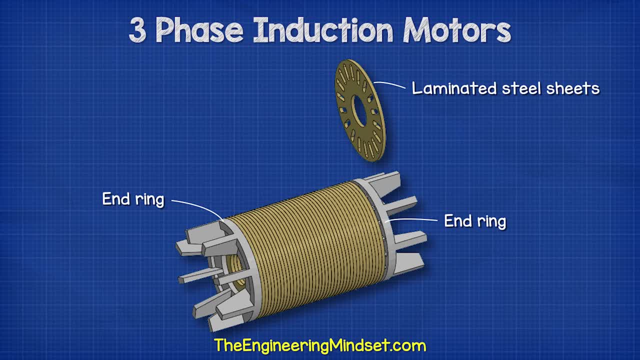 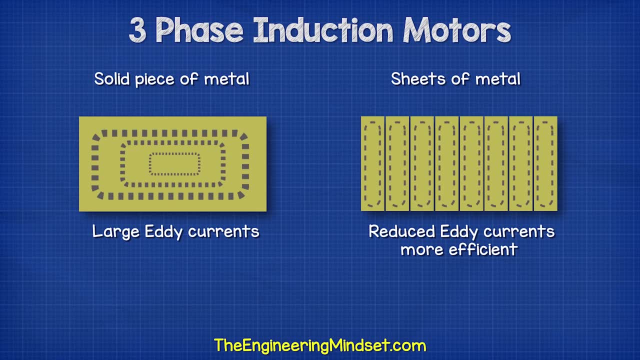 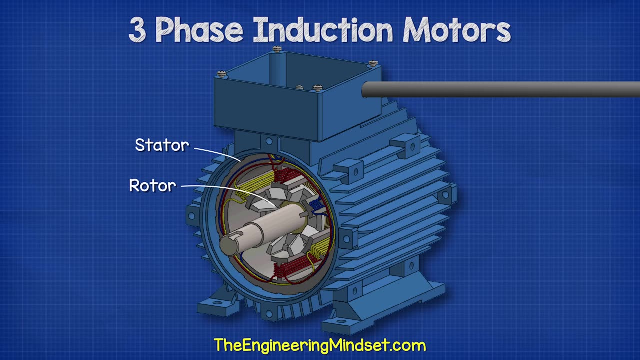 These sheets will help concentrate the magnetic field into the bars. Sheets are used instead of a solid piece of metal, as this improves the efficiency by reducing the size of the eddy currents in the rotor When the rotor is placed inside the stator and the stator is connected to. 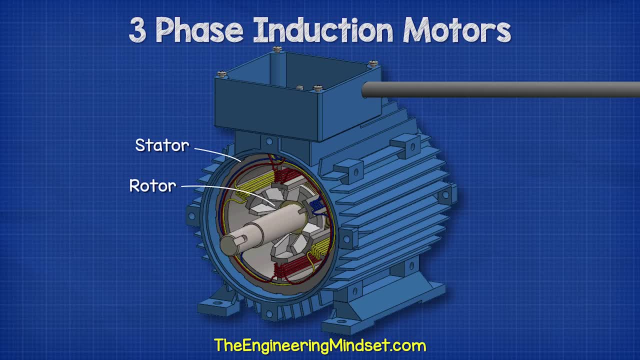 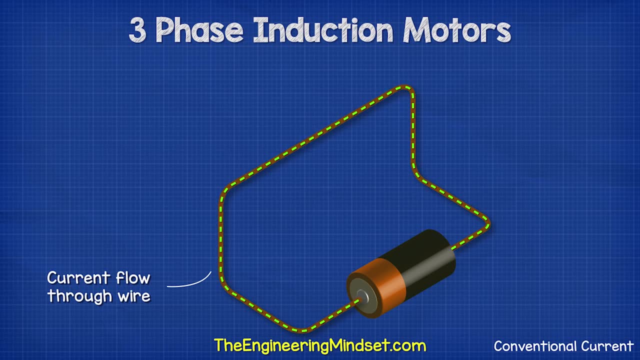 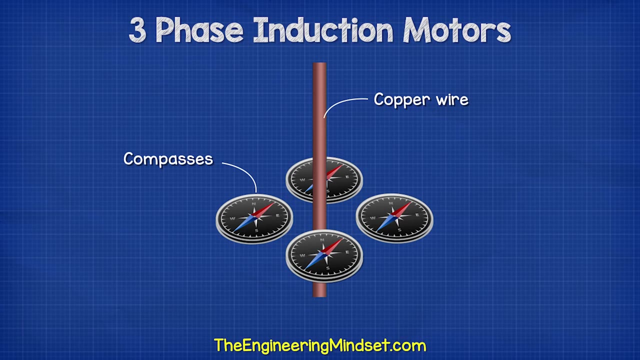 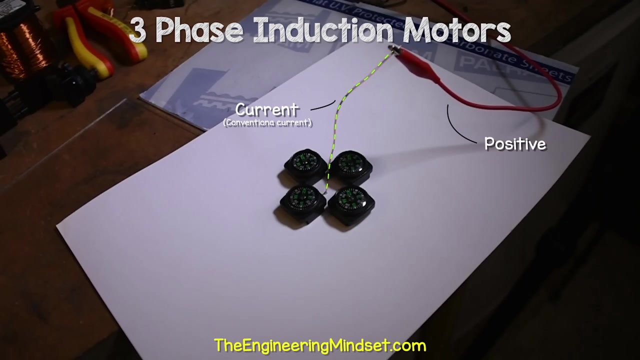 an electrical power supply, the rotor will begin to rotate. So how does this work? When electricity passes through a wire, an electromagnetic field is generated around the wire. We can see this by placing some compasses around the wire. The compasses will rotate to align with this magnetic field. If the direction. 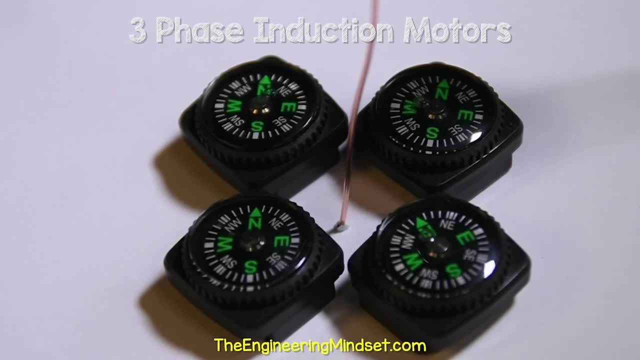 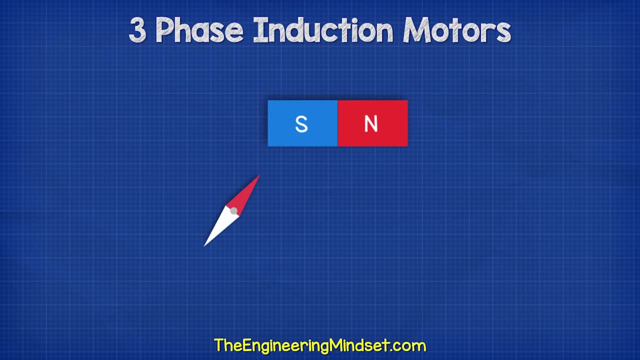 of current is reversed, the magnetic field also reverses, and so the compasses will change direction. The magnetic field of the wire is pulling and pushing the compass dials, Just like if we slide two bar magnets towards each other. It will either be attracted or repelled. We can even use one magnet to rotate another. 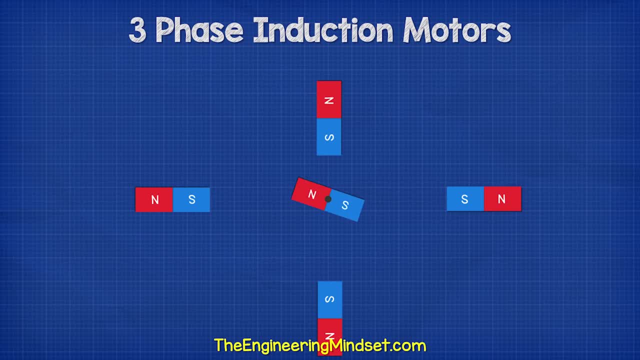 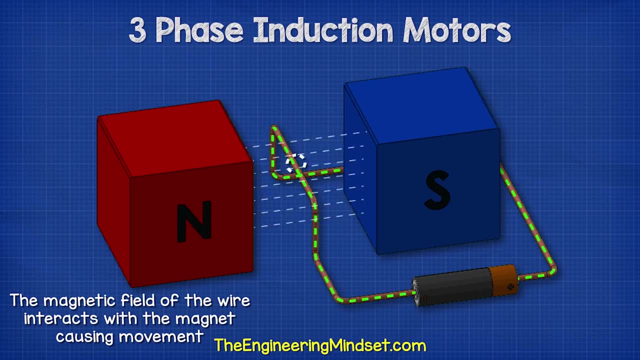 Or we could also rotate the magnet by changing the intensity of the magnetic field around it. If we place a wire in a magnetic field and pass a current through it, the magnetic field of the wire will interact with the permanent magnet's magnetic field and the wire will therefore experience a force. This force will move the wire to the magnetic field. 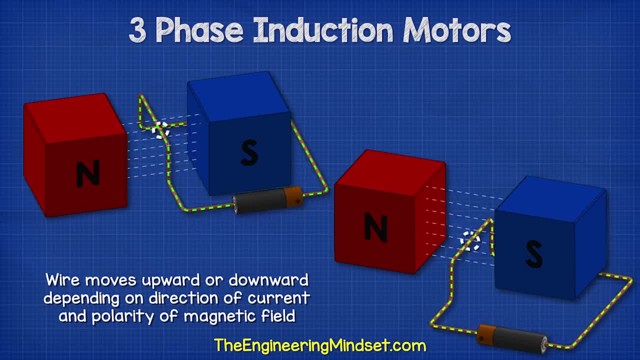 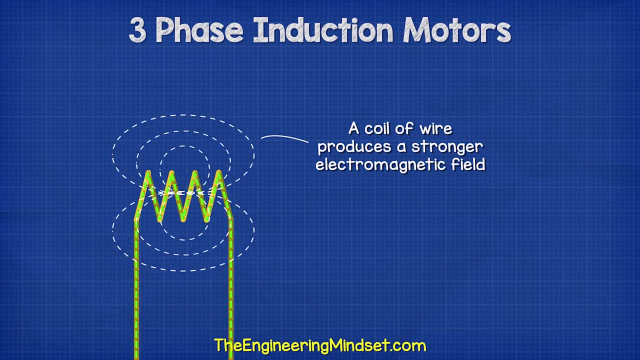 This force will move the wire either upwards or downwards, depending on the direction of current and the polarity of the magnetic fields. If we wrap the wire into a coil, the electromagnetic field becomes stronger. The coil will produce a north and south pole, just like a permanent magnet. 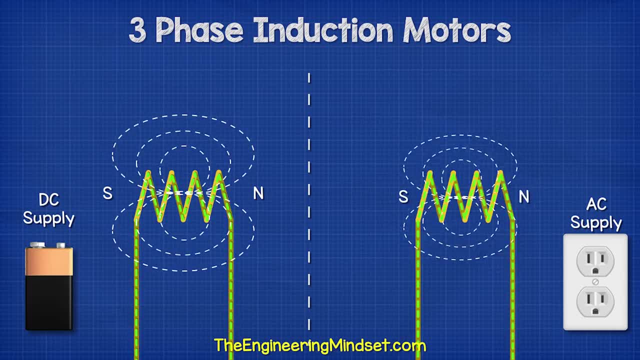 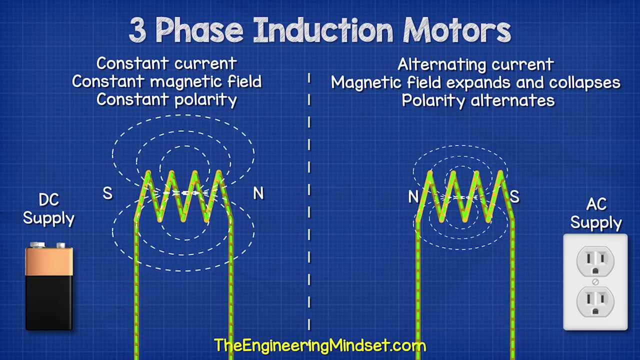 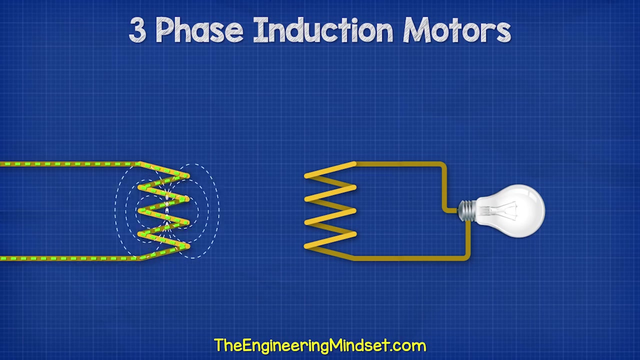 We call these coils of wire an inductor. When we pass an alternating current through the wire, the electrons will be constantly changing direction between flowing forwards and backwards. So the magnetic field will also expand and collapse and the polarity reverses each time When we place another separated coil in close proximity and complete the circuit. 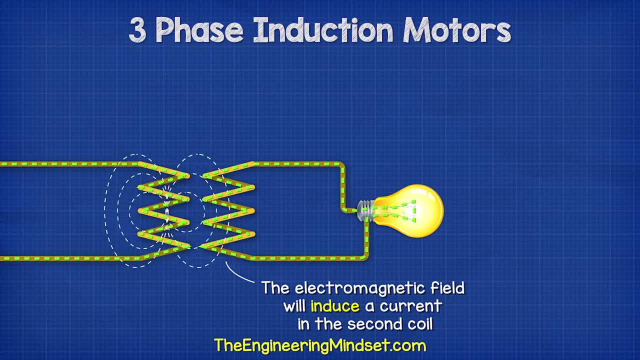 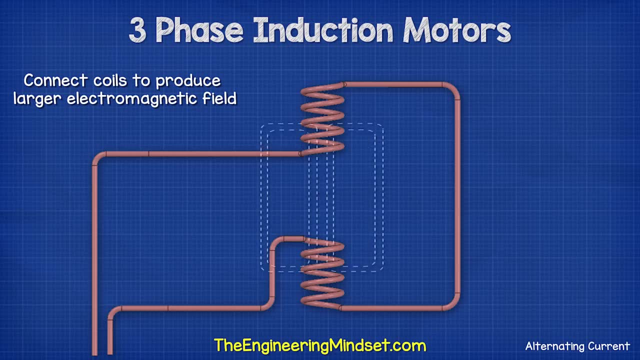 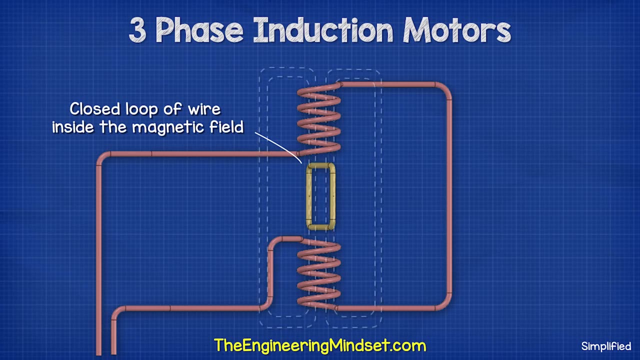 the electromagnetic field will induce a current in the second coil. We can connect two coils together and place them opposite each other to create a larger magnetic field. If we placed a closed loop wire inside this large magnetic field, we will induce a current in the loop. 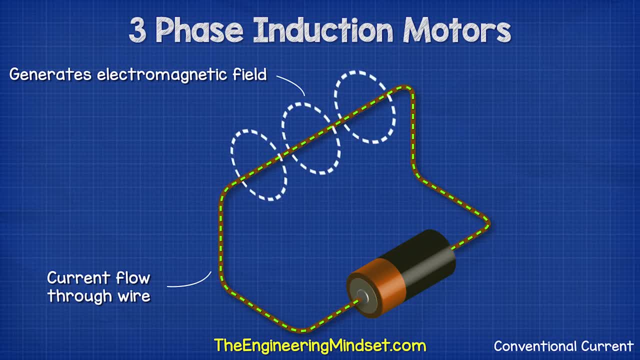 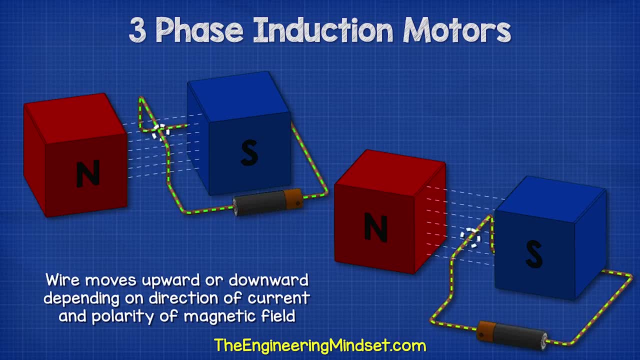 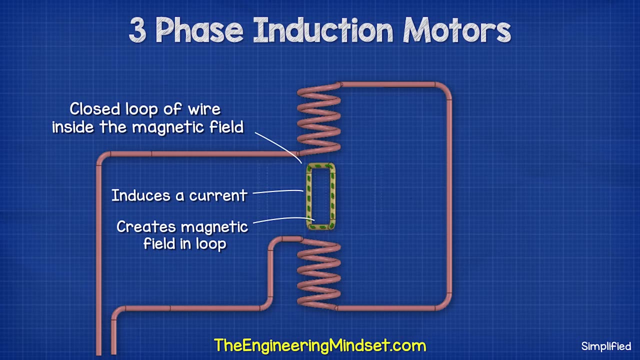 As we know, when we pass a current through a wire, it generates a magnetic field, and we also know the magnetic fields will push or pull each other when they interact. So this loop of wire will also generate a magnetic field and this will interact with the larger magnetic field. Each side of the coil will experience opposing forces, which causes it to 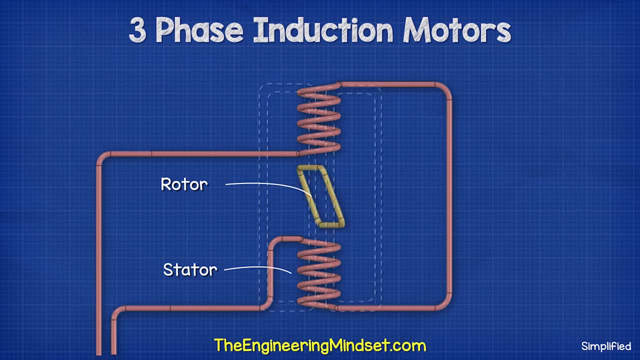 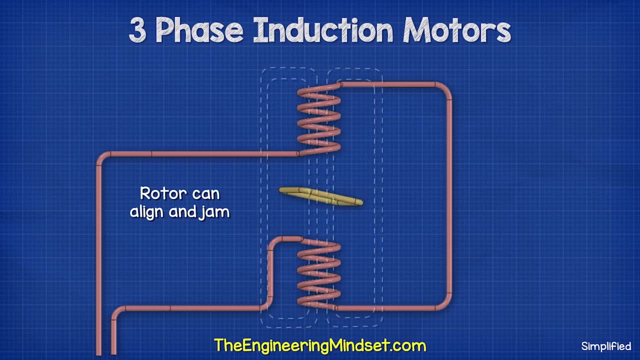 rotate. This loop is therefore our rotor and the coils are therefore our stator. The rotor will only rotate until it aligns with the stator coils. At this point it will likely get stuck as the induced current reverses with the coil. To overcome this, we need to introduce another set of coils in. 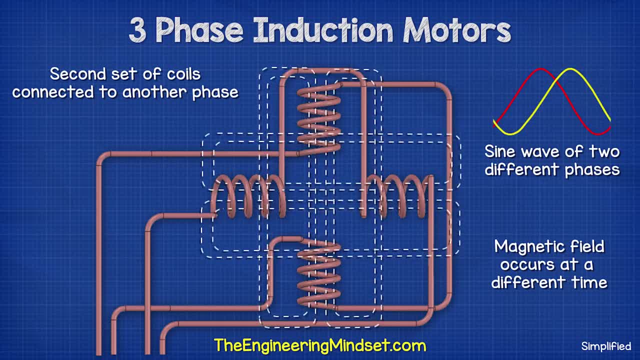 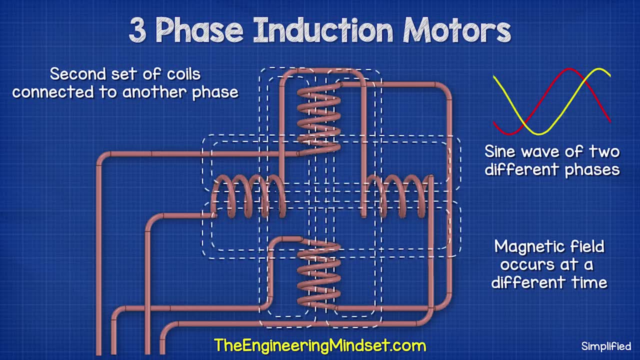 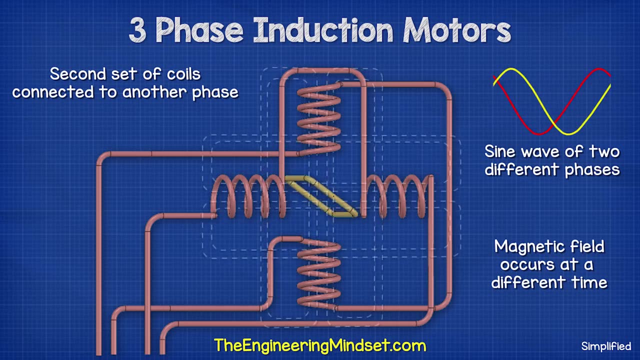 the stator and we must connect these to another phase. The electrons flow in this phase at a slightly different time, so the electromagnetic field will also therefore change in strength as well as polarity at a slightly different time. This will force the rotor to rotate Inside the 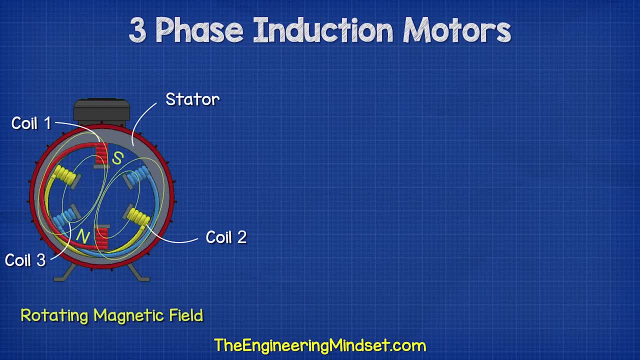 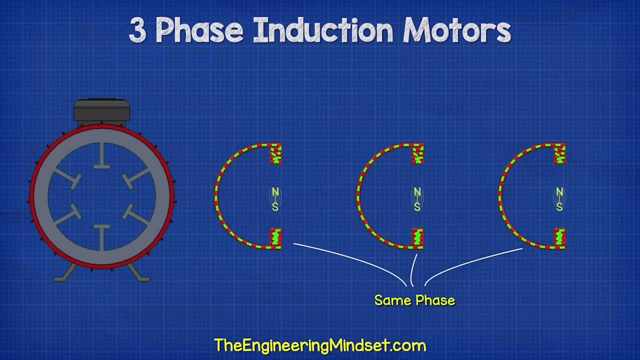 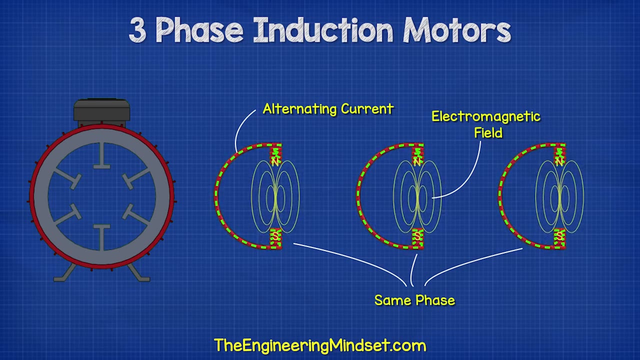 induction motor. we have three separated coils which are used to produce a rotational electromagnetic field. When we pass an alternating current through each coil, the coils will produce an electromagnetic field which changes in intensity as well as polarity as the electrons change direction. But if we were to connect each coil, 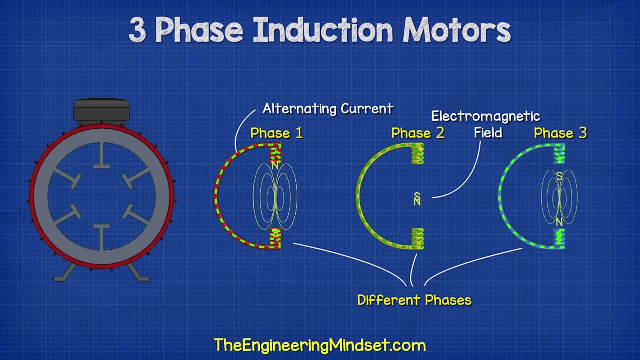 to a different phase, then the electrons in each coil will change direction at a different time. This means the polarity and intensity of the magnetic field will also occur at a different time. To distribute this magnetic field we need to rotate the coil sets 120 degrees from the 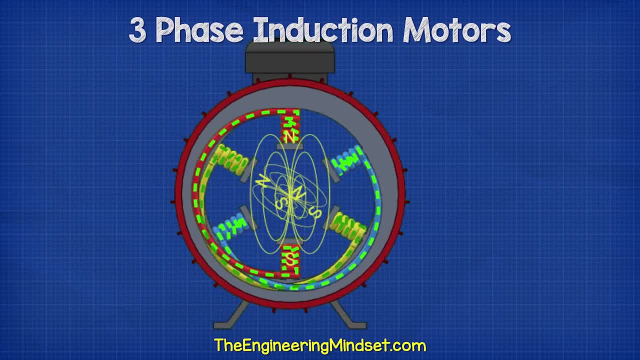 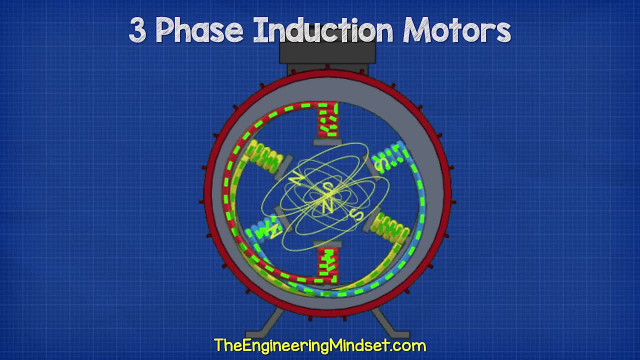 previous phase. We then combine these in a magnetic field and we get a magnetic field into the stator. The magnetic field varies in strength and polarity between the coils, which combine to produce the effect of a rotating magnetic field We saw earlier in this video. 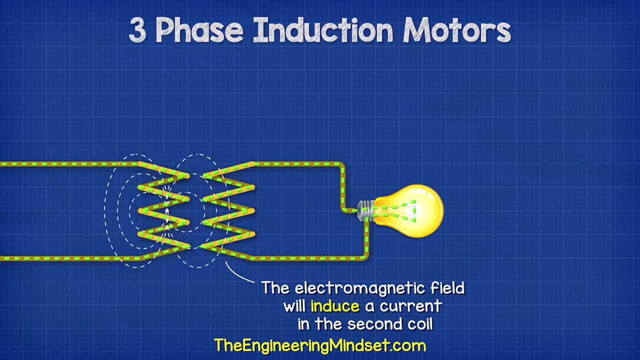 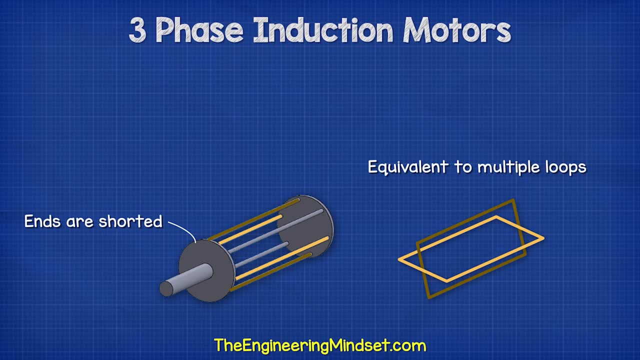 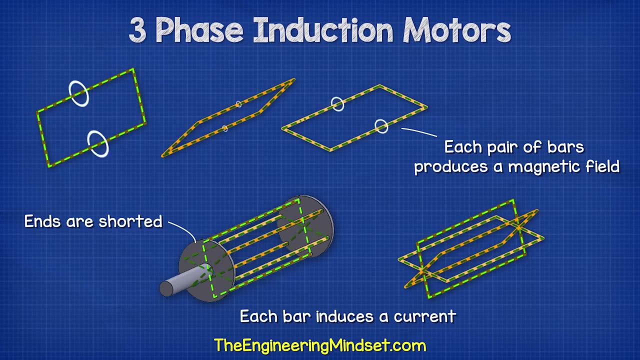 that current can be induced into a second coil when, in close proximity, The bars of the squirrel cage are shorted at each end, which therefore creates multiple loops or coils. Each bar therefore induces a current and creates a magnetic field. The magnetic field of the rotor bars interacts with the magnetic field of the stator. 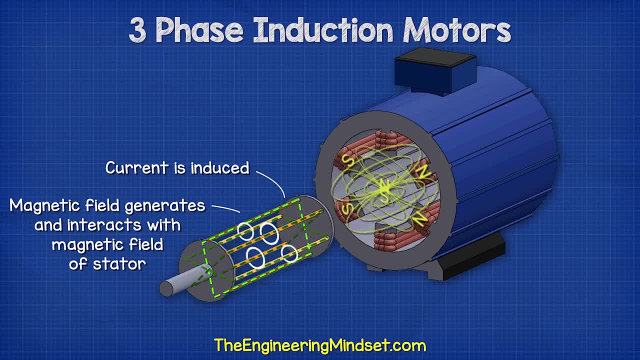 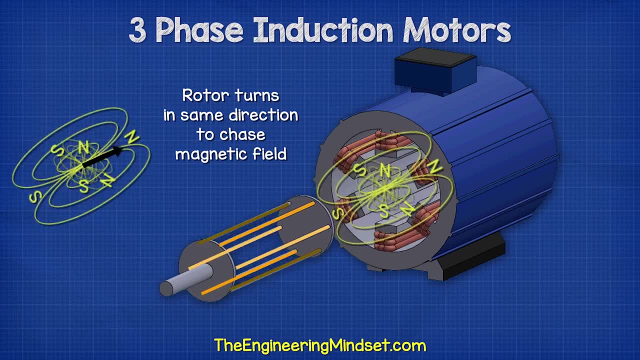 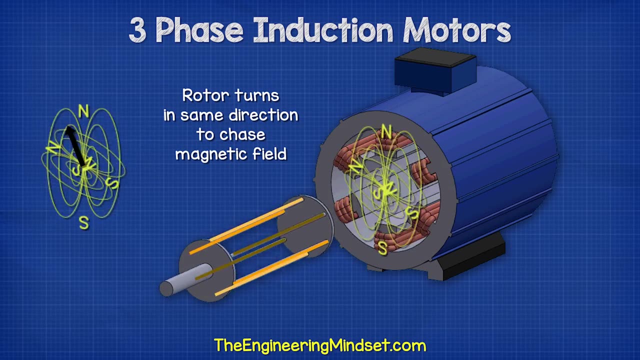 The rotor bars magnetic field is attracted to the magnetic field of the stator. As the magnetic field is rotating, the rotor will therefore also rotate in the same direction as the magnetic field to try and align with it, but it will never be able to fully catch. 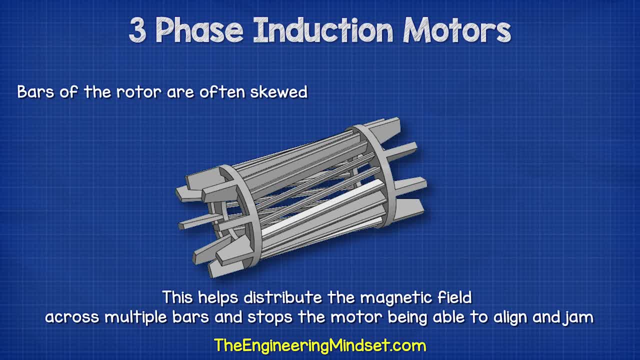 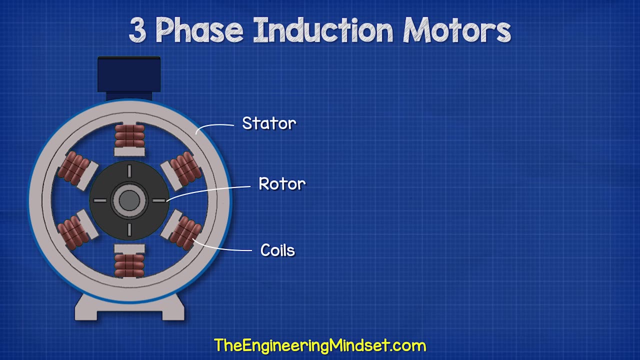 up. The bars of the rotor are often skewed. This helps distribute the magnetic field to the stator, the magnetic field across multiple bars, and stops the motor being able to align and jam. The stator contains all of the coils or windings used to create the rotating electromagnetic field. 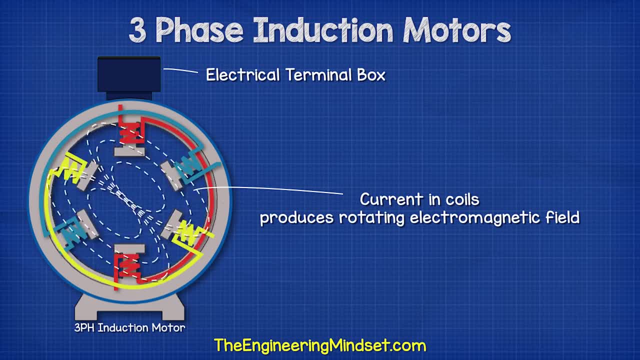 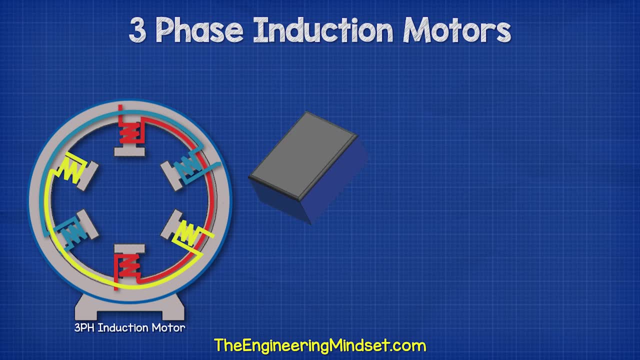 when electricity is passed through the wires To power the coils. we find an electrical terminal box on the top or sometimes on the side. Inside this box we have six electrical terminals. Each terminal has a corresponding letter and number. We have U1, V1 and W1, then W2, U2 and V2.. 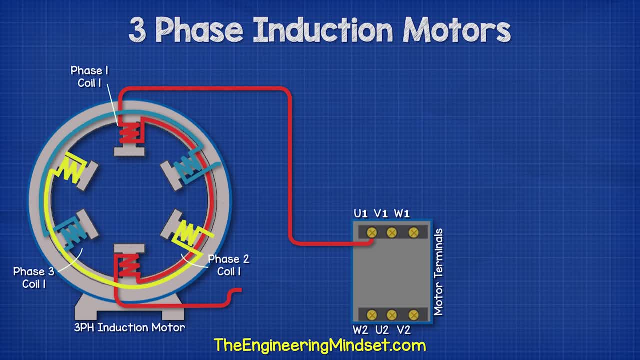 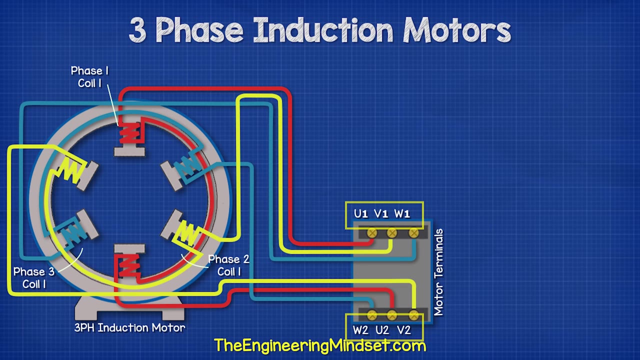 We have our phase 1 coil connected to the two U terminals, then the phase 2 coils which are connected to the two V terminals, and lastly the phase 3 coil which is connected to the two W terminals. Notice that the electrical terminals are arranged in a straight line. 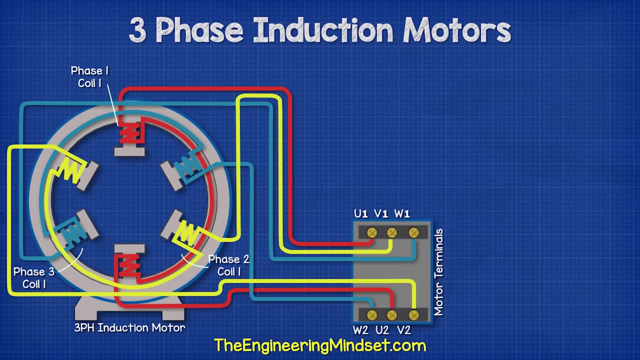 They are arranged in a different configuration on one side to the other. We will see why that is in just a moment. We now bring in our three phase power supply and connect these to their respective terminals. For the motor to run, we need to complete the circuit, and there are two. 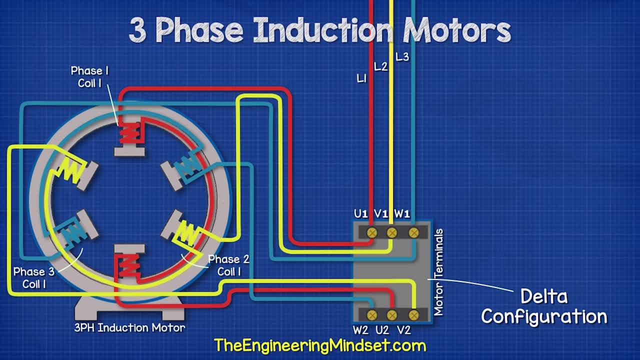 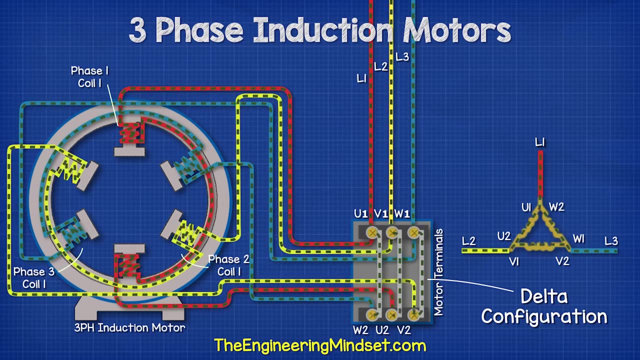 ways to do this. The first way is the delta configuration. For this we connect across the terminals U1 to W2, V1 to U2 and W1 to W2.. This will give us our delta configuration. Now, when we provide AC current through the phases, 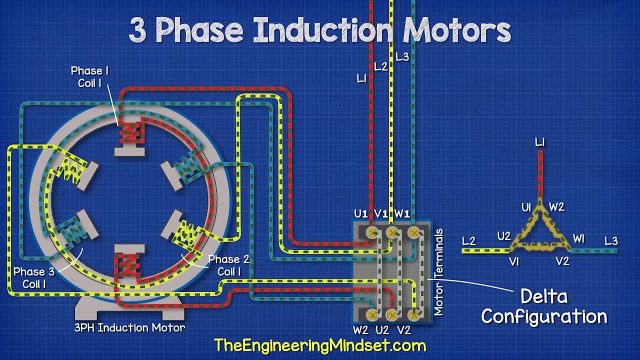 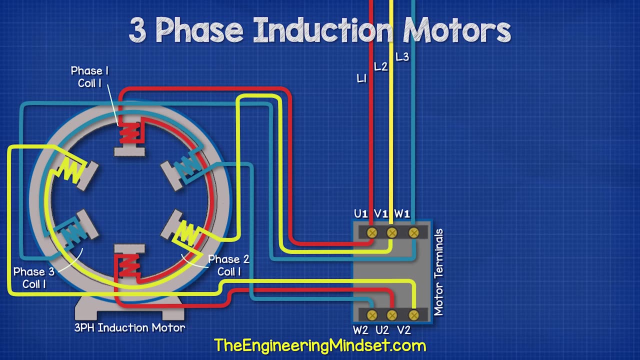 we see that electricity flows from one phase to another as the direction of AC power reverses in each phase at a different time. That is why we have the terminals in different arrangements in the terminal box, Because we can easily connect across and allow electricity to flow. 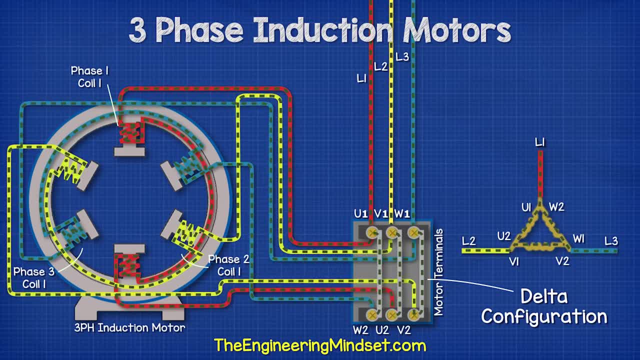 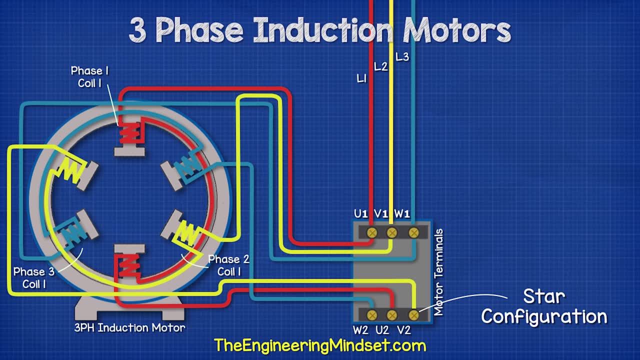 between the phases, as the electricity flows from one phase to the other. The other way we can connect the terminals is to use the star or Y configuration. In this method, we connect between W2, U2 and V2 on only one side. This will give us our star or Y equivalent. 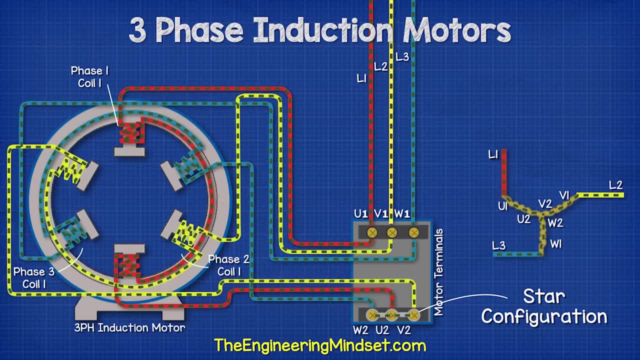 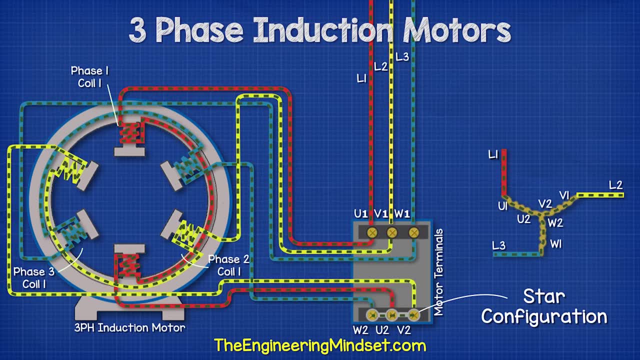 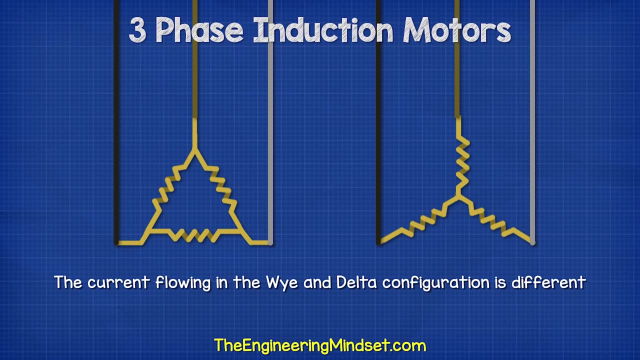 connection. Now, when we pass electricity through the phases, we see the electrons are shared between the terminals of the phases Due to their design differences. the amount of current flowing in the star and delta configuration is very different and we're going to see some calculations for these towards the end of this. 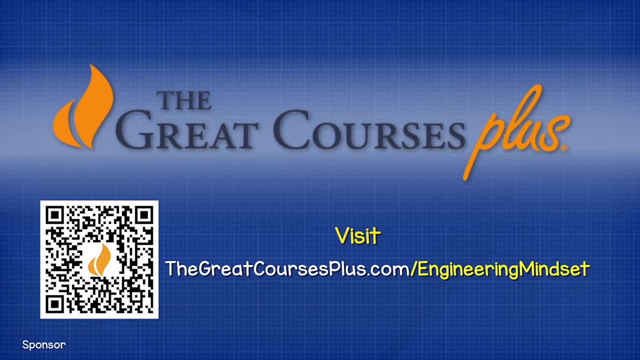 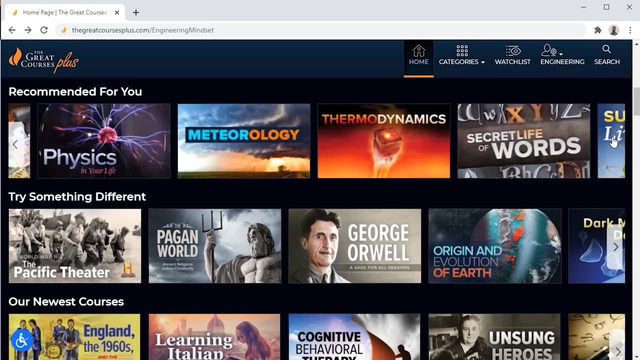 video. But first I want to tell you about The Great Courses Plus. All of our viewers can get a free trial right now by visiting thegreatcoursespluscom. forward slash engineering mindset. The Great Courses Plus is an on-demand learning platform that lets you binge watch. 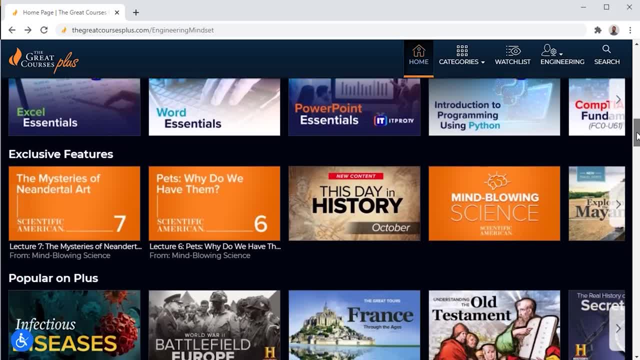 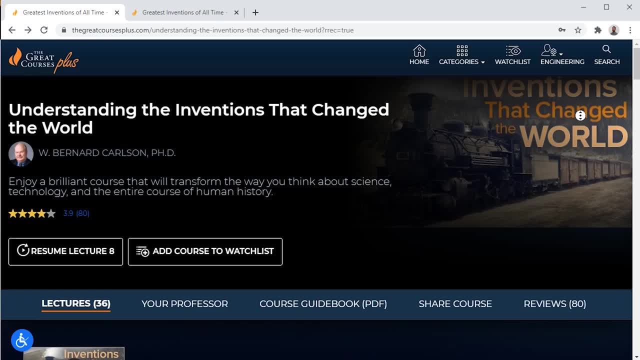 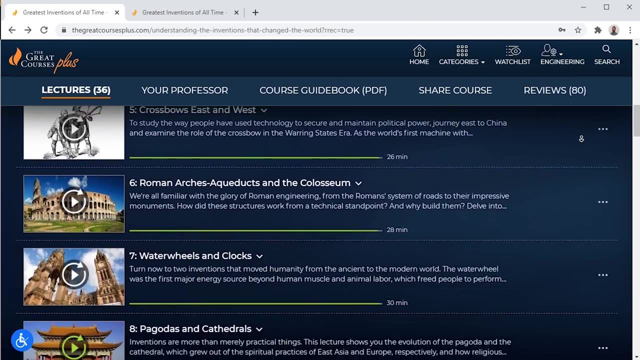 courses. They have over 13,000 videos by industry experts on everything from science, maths, history and even cooking. Personally, my favourite is their engineering lectures and their course on inventions that change the world. As a fan of this channel, I'm certain you'll also find these. 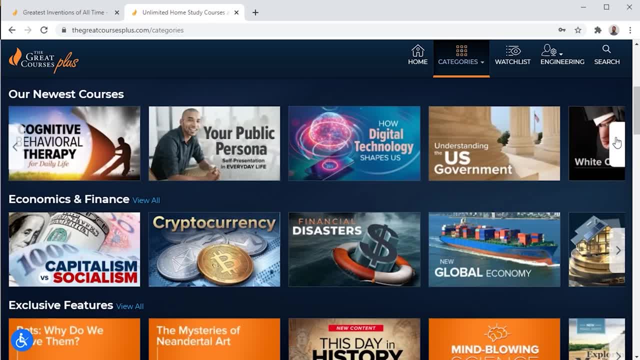 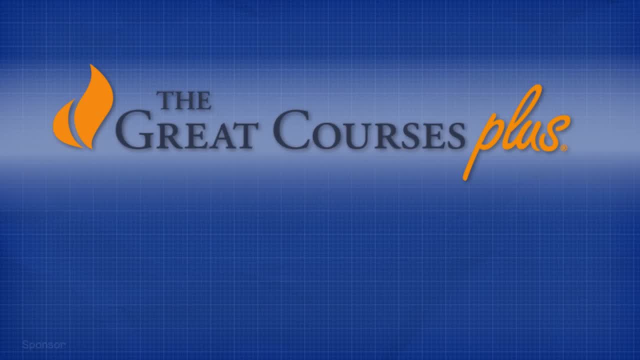 interesting too, so do check those out. They add new content every month and you can watch as many videos as you want from your TV, tablet, laptop or phone. Just click the link in the video description down below to start your free trial today. 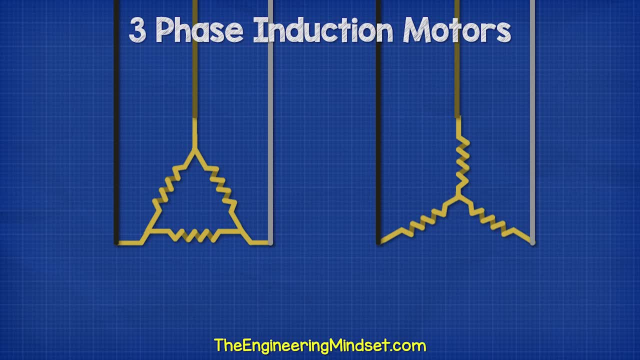 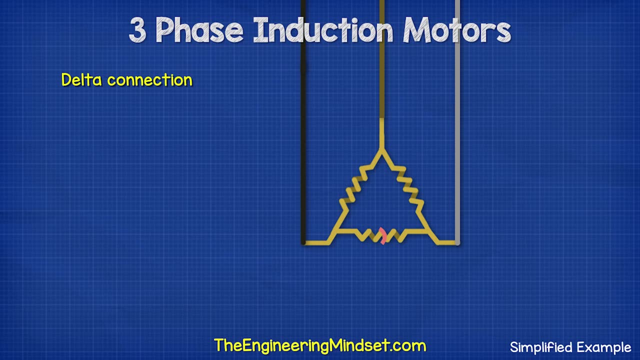 Let's have a look at the difference between the star and delta configurations. Let's say we have the motor connected in delta with a supply voltage of 400 volts. That means when we use a multimeter to measure the voltage between any two phases, we will 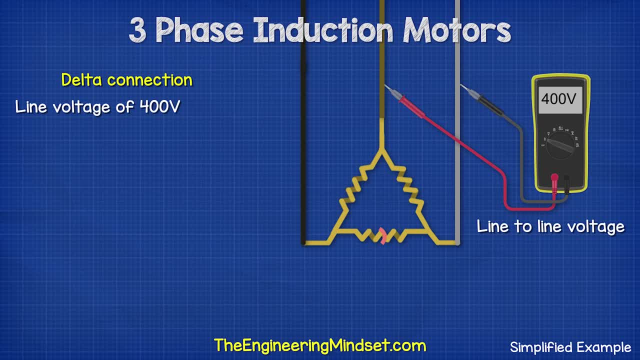 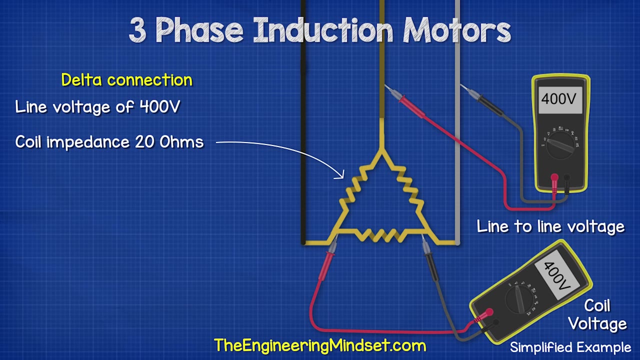 get a reading of 400 volts. We call this our line to line voltage. Now if we measure across the two ends of a coil, we again see the line to line voltage of 400 volts. Let's say each coil has a resistance or impedance. as this is alternating current, 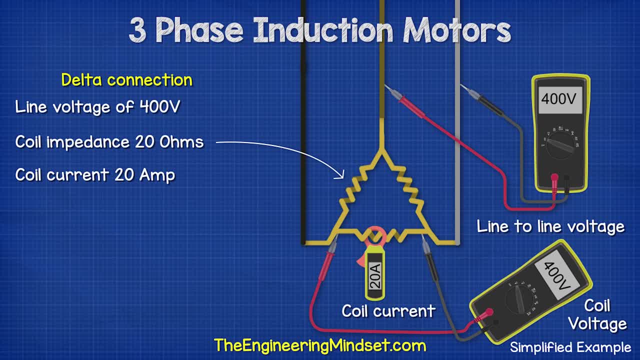 of 20 ohms. That means we will get a current reading on the coil of 20 amps. We can calculate that from 400 volts divided by 20 ohms, which is 20 amps, But the current in the line will be different. It will be 34.6 amps. We get that from 20 amps multiplied by the square. 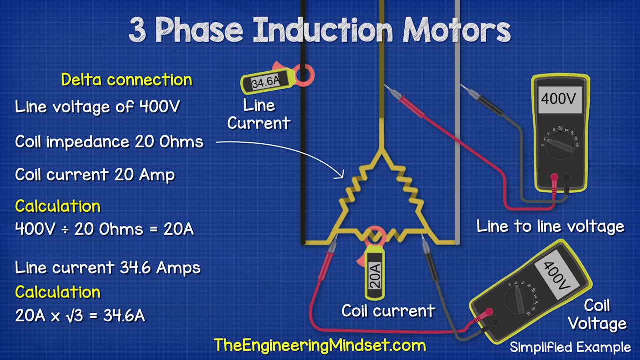 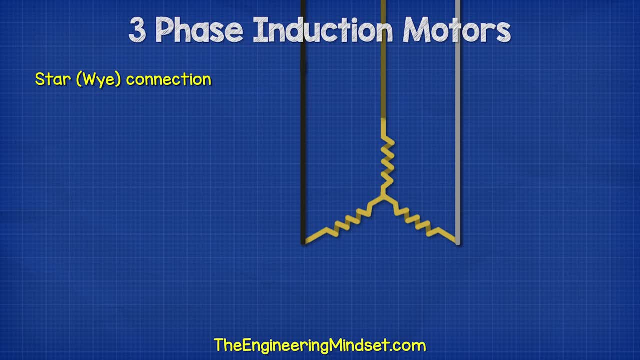 root of 3, which is 34.6 amps. That's because each phase is connected to two coils. Now if we look at the star or wire configuration, we again have a line to line voltage of 400 volts. We see that if we measure between any two phases.